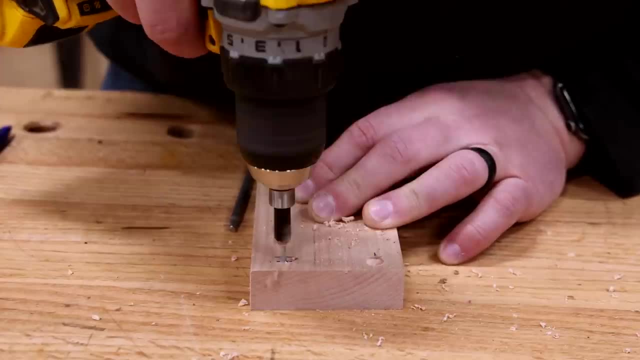 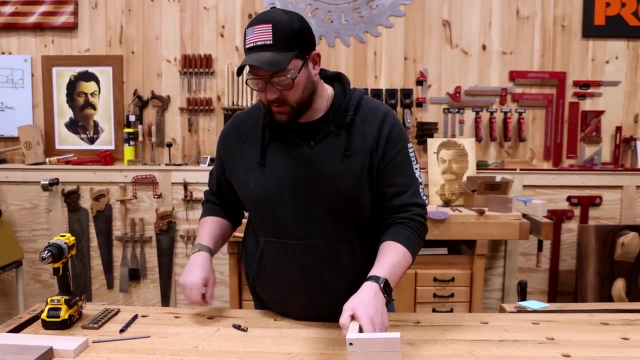 own. This tool makes it super easy. Here we've got a butt joint. We've got two super ugly looking screw holes on the outside here. but I'm smart so I know that that hole is 3-8ths of an inch and I also know that this plug cutter is also 3-8ths of an inch And we're 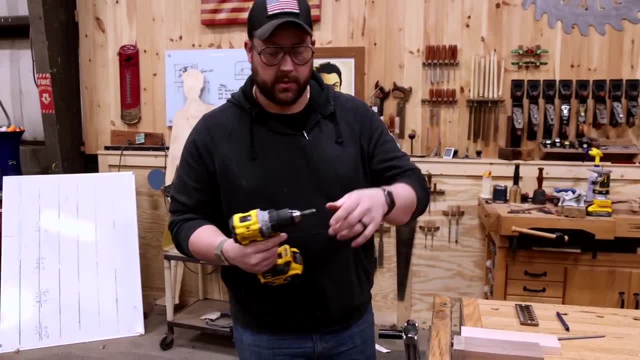 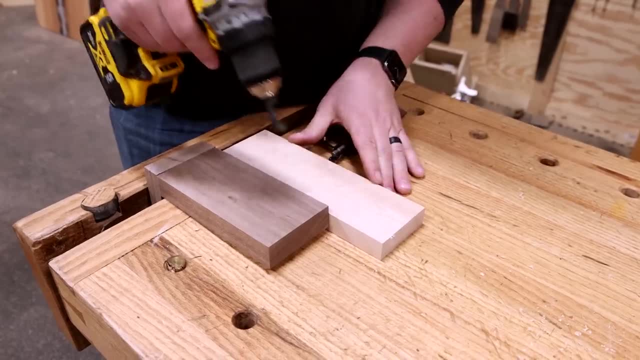 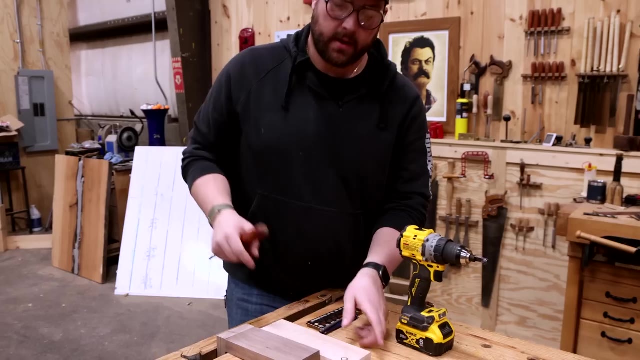 going to put it in a handheld drill, because we're only cutting one. but usually you want to use a drill, The dowel press. it lets you cut plugs to match or to contrast. So here we've got some maple, but I can just come on in and cut a maple plug. that's literally made out. 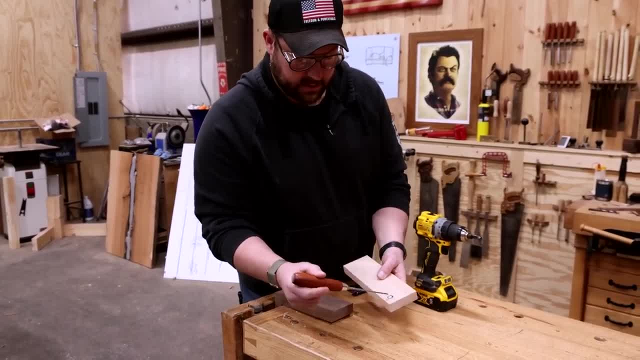 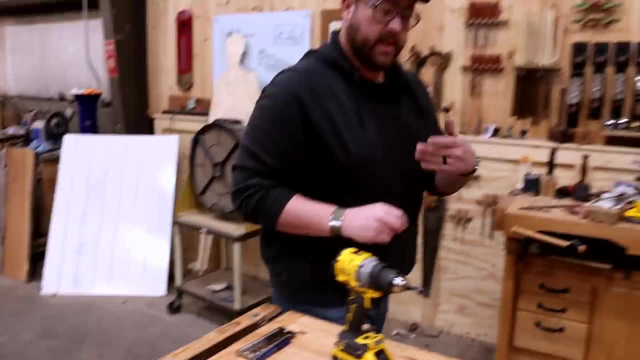 of the same material as the other end of the board that we just made that joint out of. This is great for, like drawer boxes and, honestly, any joinery where you're going to be face jointing something All you do. now add yourself a little bit. 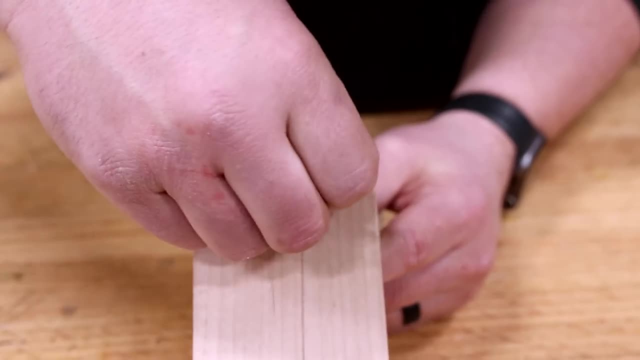 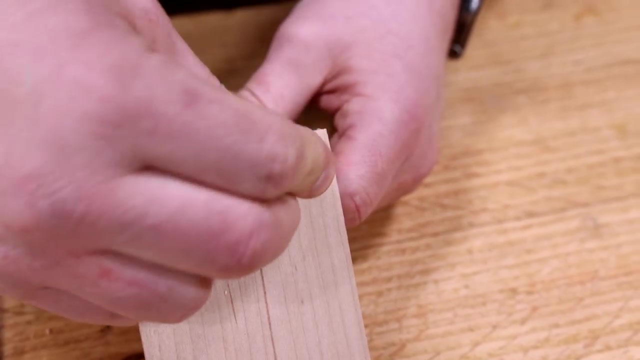 of glue to the joint, Put your plug in And if you want to go more professional, you can match the grain Which. this grain is going this way and obviously that joint is going that way. Let that set up a little bit And in the meantime we're going to drill a contrasting 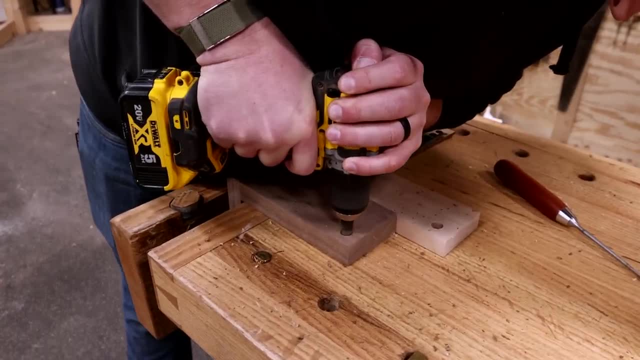 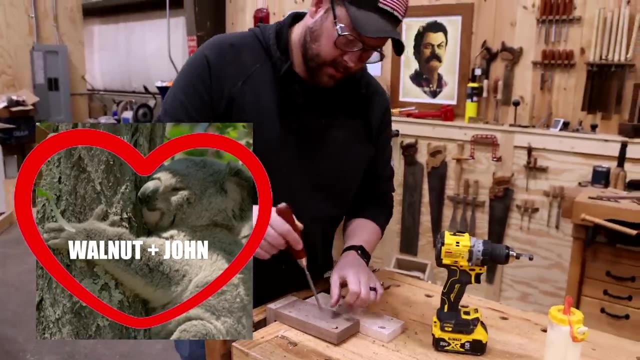 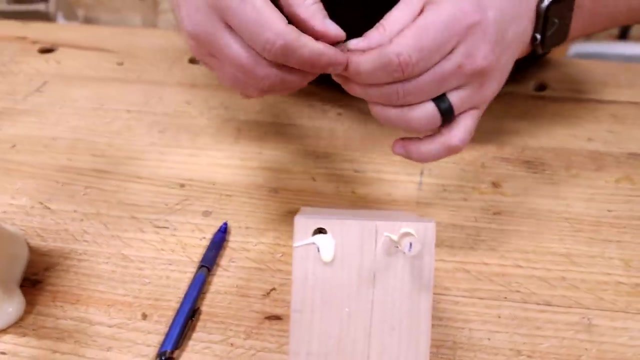 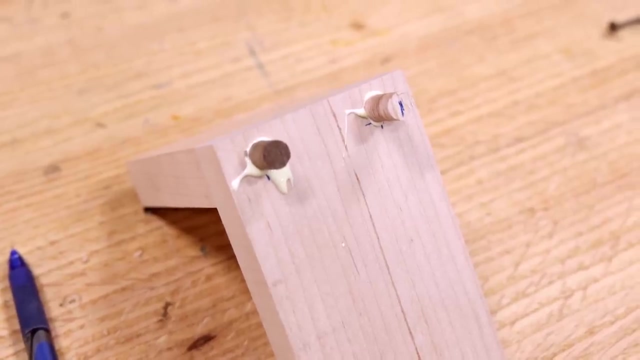 one out of some walnut, Which I tend to be a huge fan of because I think the contrasting plugs are super rad and add a lot of cool contrast to the joint. So here we've got our dowel press. Same thing. That's a lot of glue. That's like way too much glue Here. 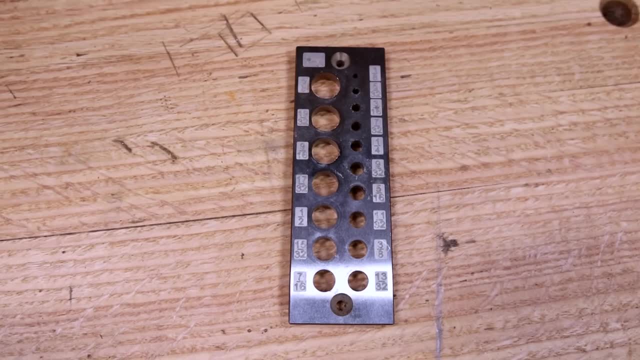 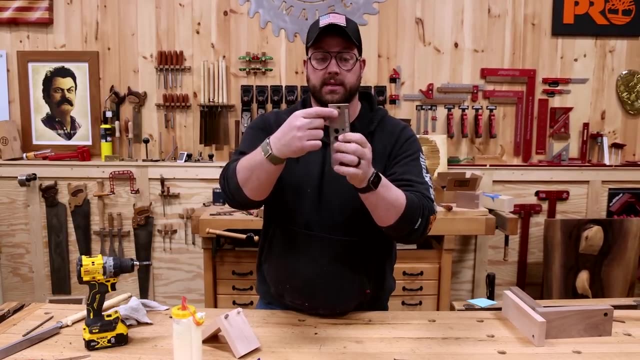 Now, while that glue sets up, I also want to make a suggestion for this dowel cutter from DFM Toolworks. I made it TikTok, as you can see right here. It's super easy. You can take stock all the way from this, which I think is 5 eighths, down to 1 eighth on here You. 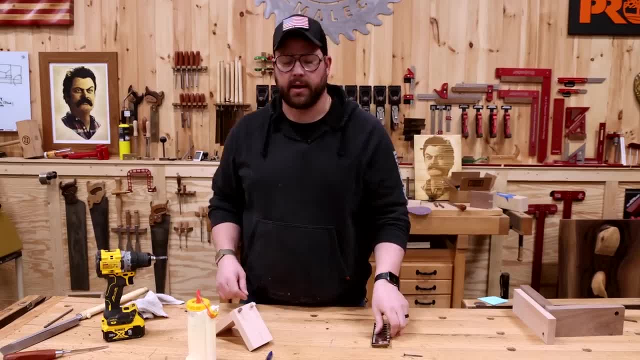 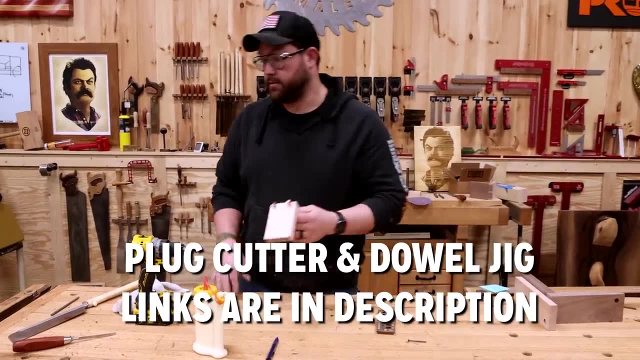 just hammer it through the hole. They sell this for about 60 bucks, and the plug cutters are dirt cheap and super easy to find at your big box store if you want to get into it. So now that these are set up a bit, let's cut them out and show you what this looks. 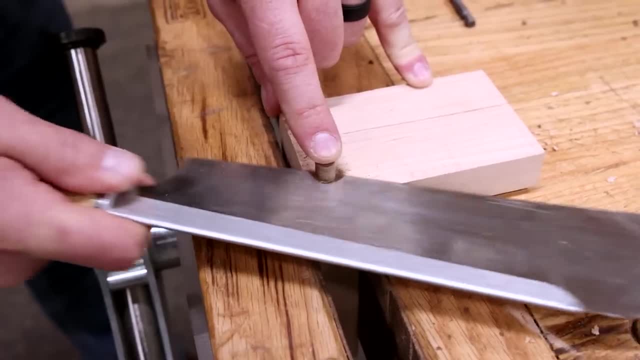 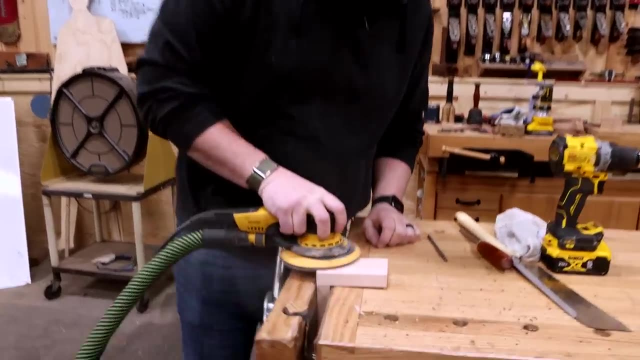 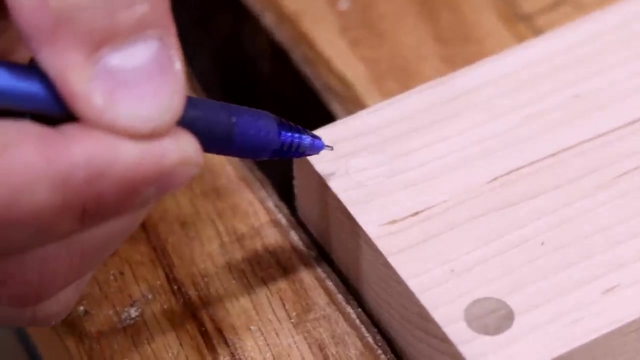 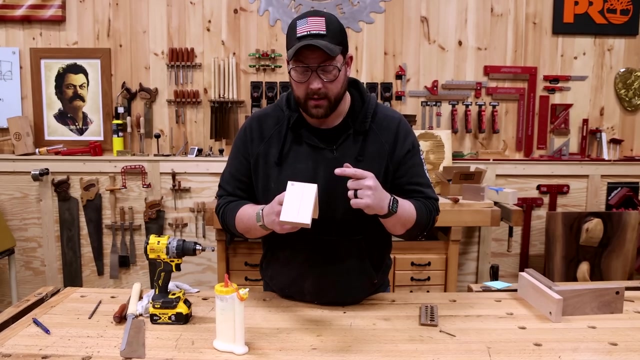 like. Now all you've got to do is sand them to look pretty. Now that maple one matched so good with the grain you can barely tell it's there, And this doesn't even have finish on it. Easy way to step up your woodworking: Add some plugs to your face screws. You can really. 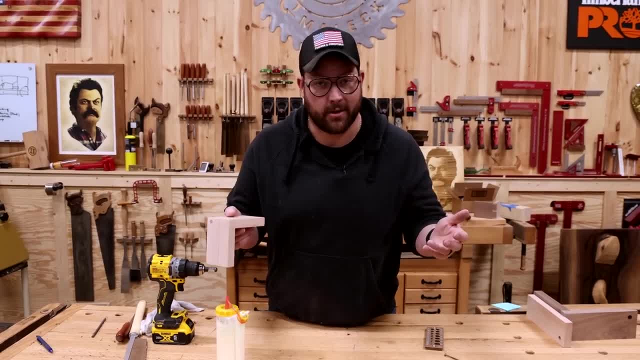 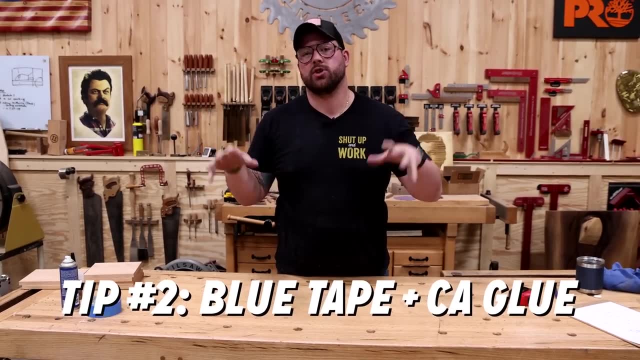 start to make things look cool and you don't have to invest in a silly pocket hole jig. Next, tip number two: It's pretty common and you've probably seen a bunch of us use it, but it is using blue tape instead of double sided tape, with the addition of CA glue. Let's 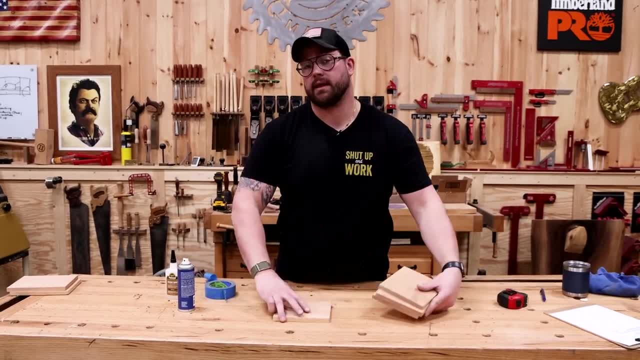 say, for instance, I have all four of these boards and I want to make them all the exact same size. Well, instead of making one and then trying to make them all the exact same size, I'm going to make them all the exact same size. 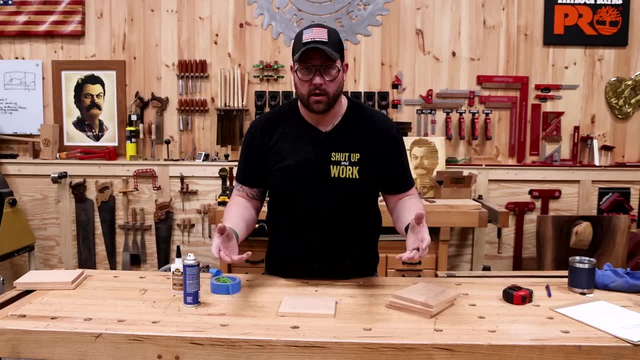 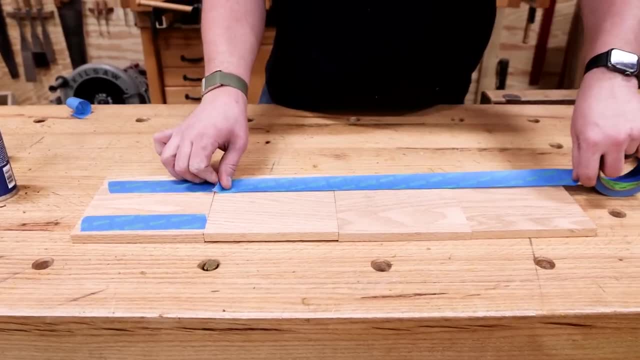 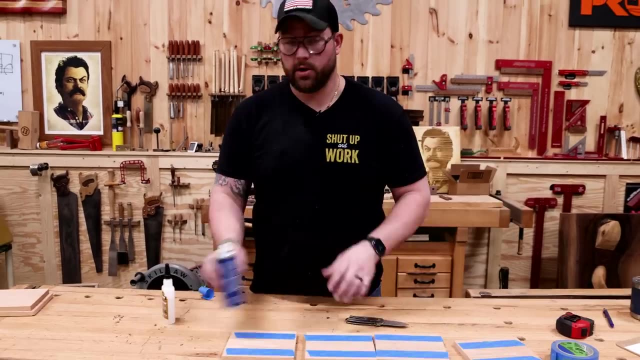 And then trying to mimic and copy all of them. we can do all of that work at once. All you've got to do is take your blue tape. you want to lay it out on the bottom of all of them in a relatively similar fashion. So here you're going to need CA glue and activator. 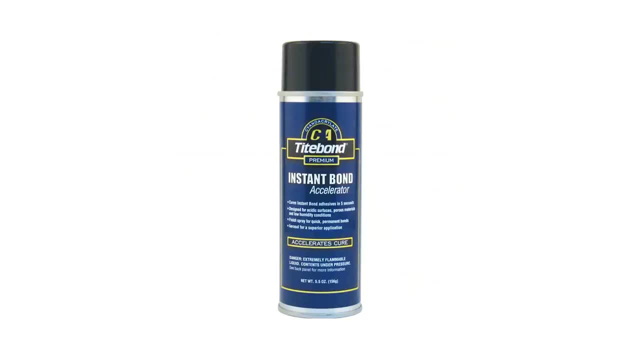 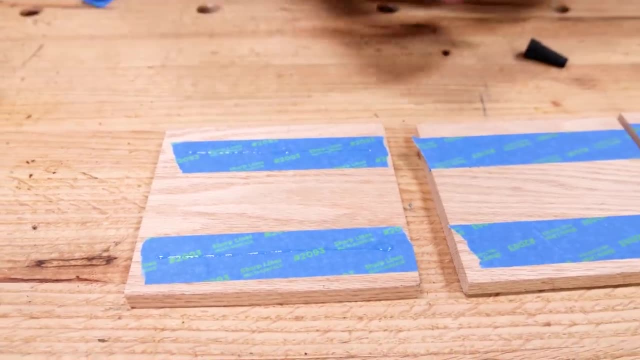 I like Titebond products, but there's a ton of other good stuff out there. This is medium. You don't want to use the thicker stuff. All you do. give yourself a line down the one piece and then, with the other piece, spray the activator on the tape. You'll flip it. 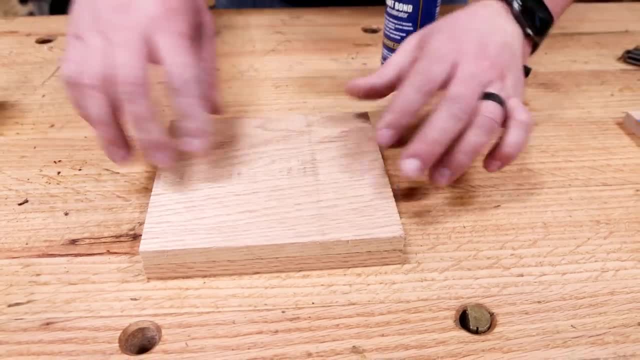 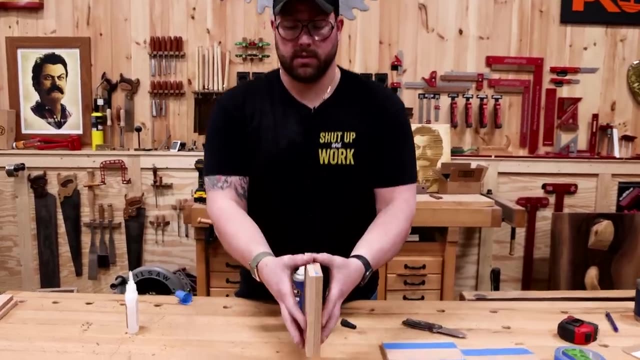 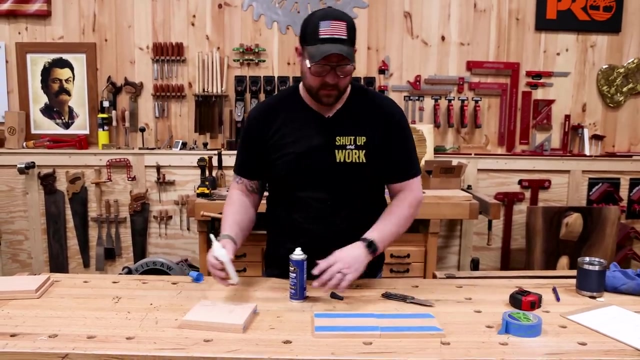 on making sure you're aligned, Get your corners and stuff aligned, Push it down, Wait a couple seconds and now these boards are stuck together, but not permanent, So we have two more over here. I'll do the same thing And then, to make it simple, I'll. 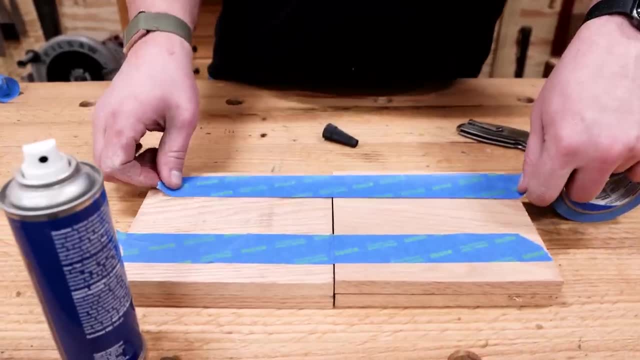 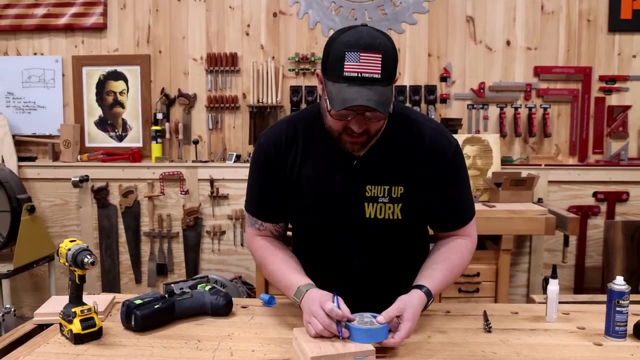 do it one more time to get all four pieces aligned. So a good example of something we like to do is say: you want to do a drawer pull right Now. all you've got to do is mark it out on this one piece and then we can cut it out. 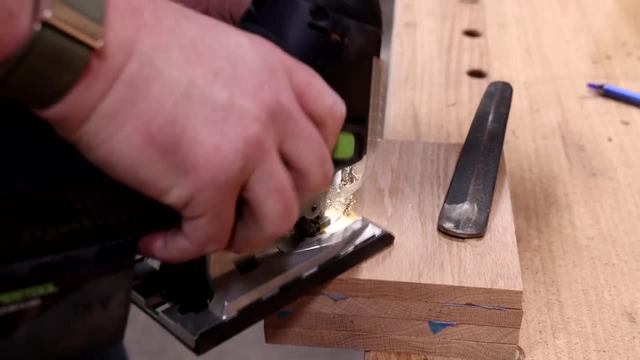 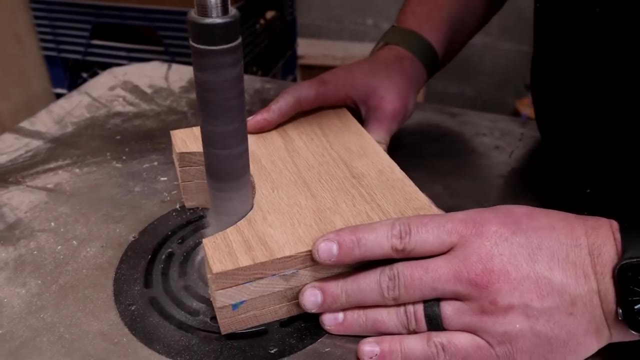 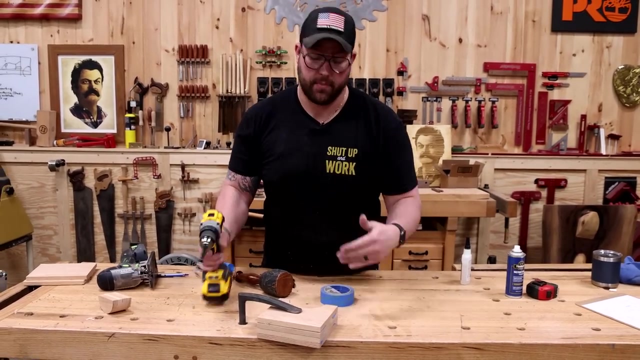 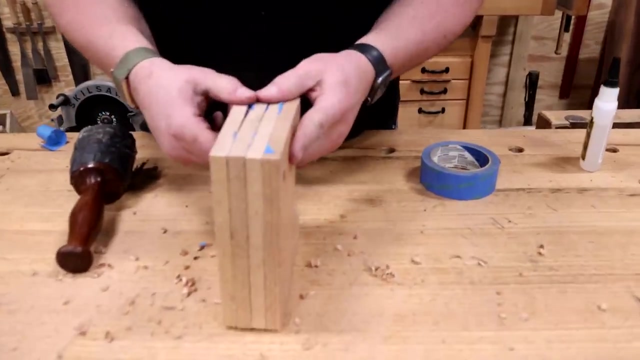 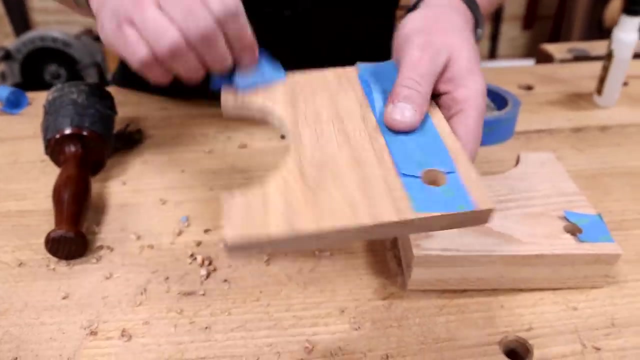 and all four pieces will be the exact same. It's also a great way if you want to drill holes in something and have them all line up or be perfect or whatever. pop them apart and you can see it leaves no residue and it's so much easier to remove than double-sided tape. Most double-sided tape is made for carpets. 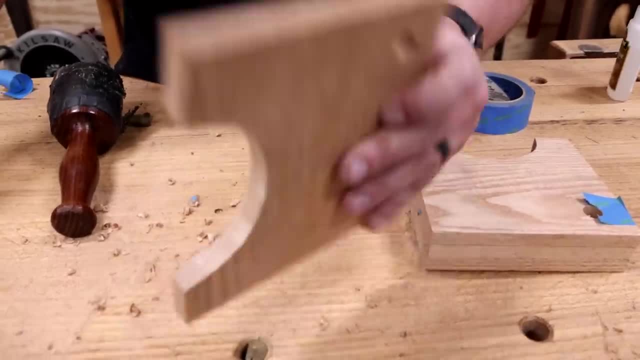 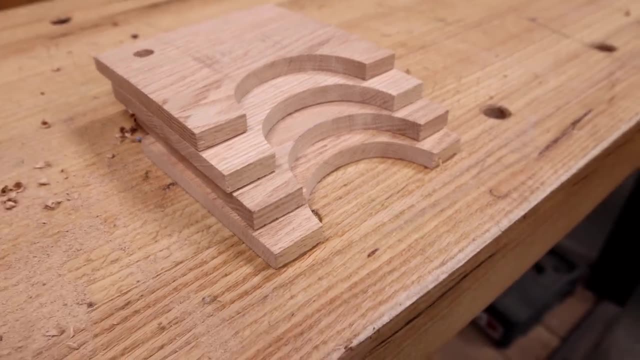 It gets really gummy, It gets really thick, but all of these parts are now going to be the exact same And it's way, way, way easier now. It's much easier and cheaper than buying double-sided tape for most applications. 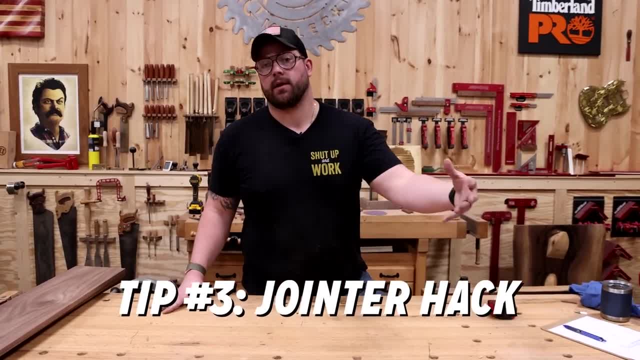 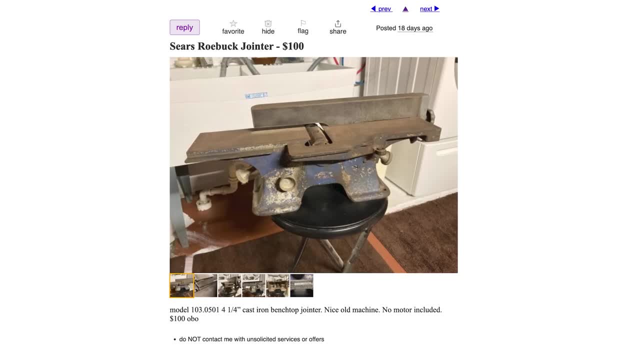 This next tip is going to be for those of you out there that have a jointer and are looking to do better tabletop glue-ups. When I got started, my first jointer was a Craigslist purchase, and it wasn't the greatest tool ever, right. 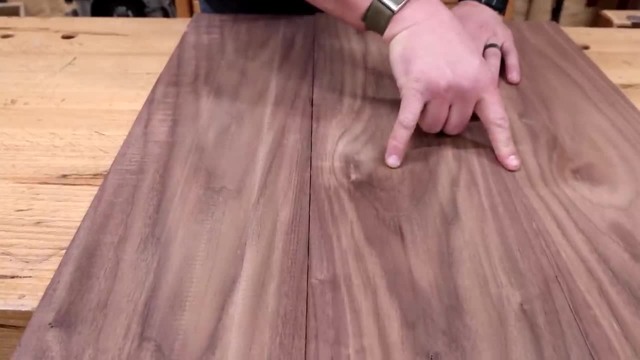 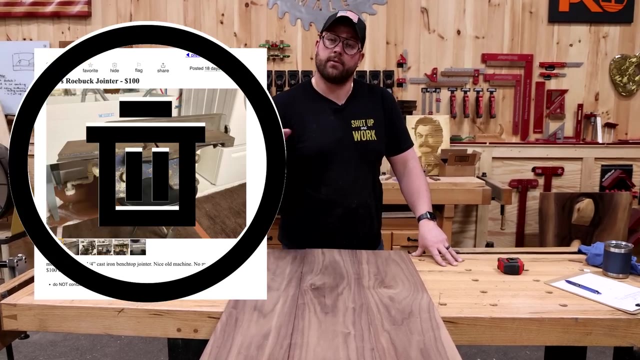 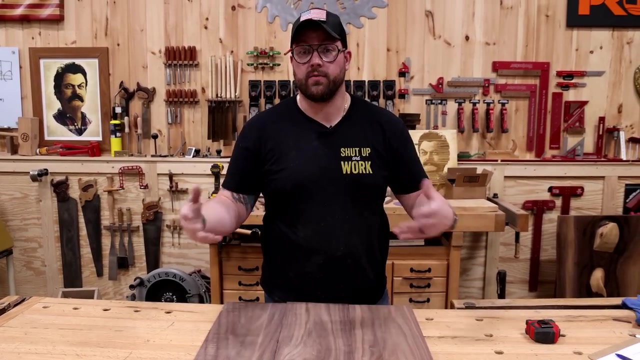 I always had issues with glue seams not being tight on my tabletops and panel gloves or whatever. I always thought the jointer was just not that good. In reality, it's really difficult to keep a jointer perfect. So this tip- regardless if your jointer is set up perfect or not- will give you a way. 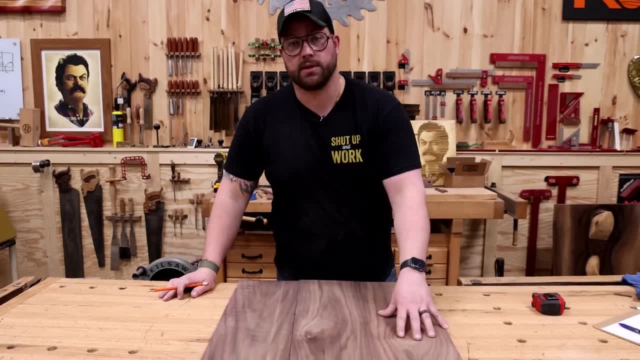 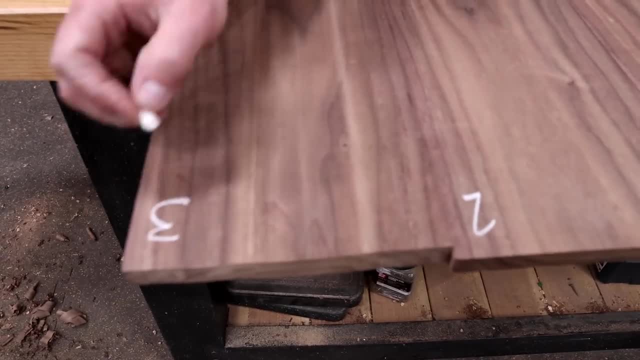 better glue-up. First thing you're going to want to do is lay out your boards in the order that you're going to be gluing them up. I like to mark mine in the corner and number them so we know one goes to two, two goes. 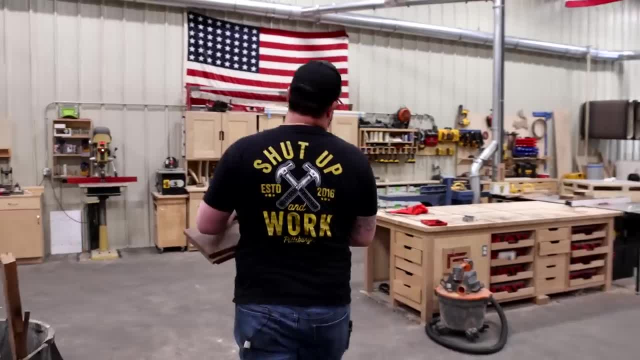 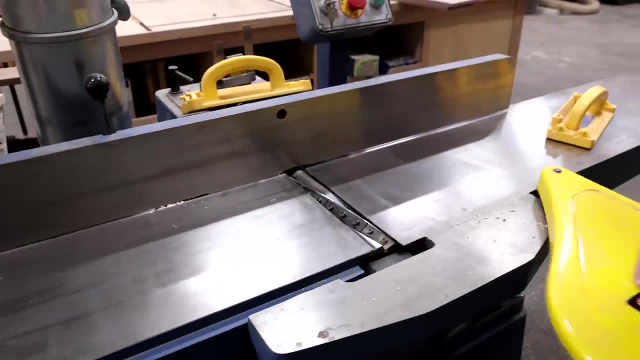 to three. Keeping it simple, Let's go over to the jointer. So this is a jointer, If you're not familiar. it makes things flat. on one side, You have a cutter head, a bed and a fence. Those are the three things I'm talking about here. 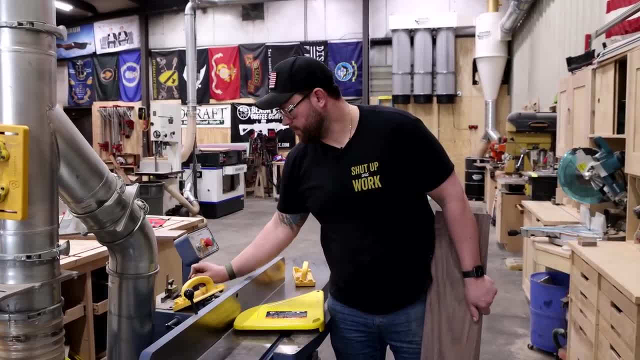 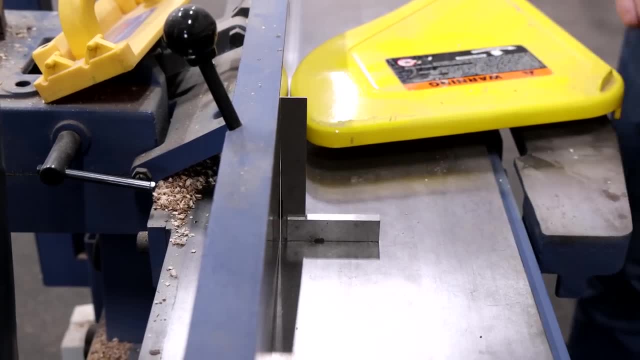 What you want to do is get your fence as close to square as possible. I keep these engineering squares on the jointer and you can see here it's just slightly out right, And so this happens from time to time and it's quite common. 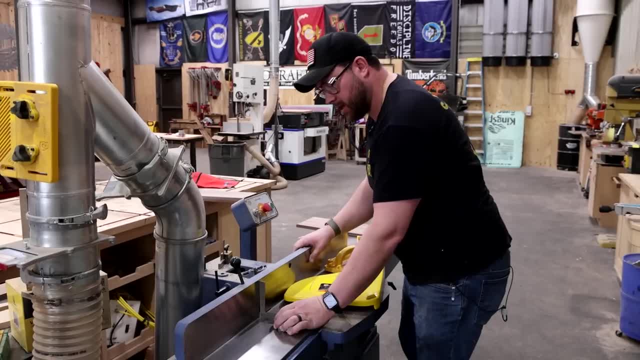 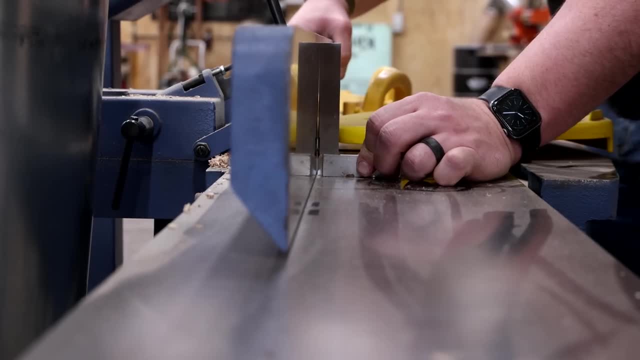 You'll try to adjust it the best that you can, but in reality it's going to come out of square more often than not. Extreme example, right, Let's move it back into square Here, And I'm actually going to leave it a little bit out to show you guys how this trick works. 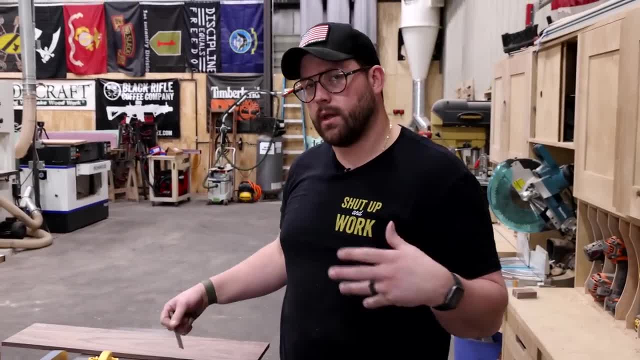 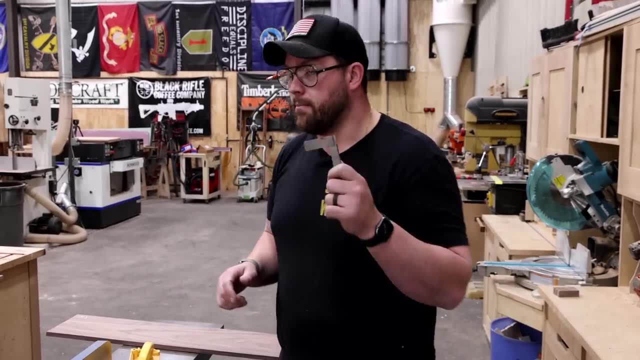 even better. When you're jointing boards, you want to joint one edge first and then rip the other edge on the table saw. Typically, this will give you a pretty solid glue up. But if you do that and you're not getting a solid glue up, that's where this trick applies. 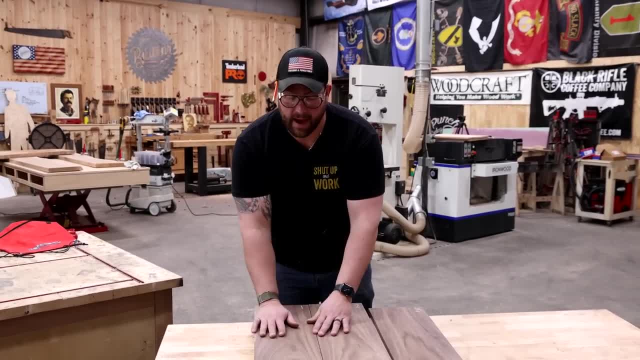 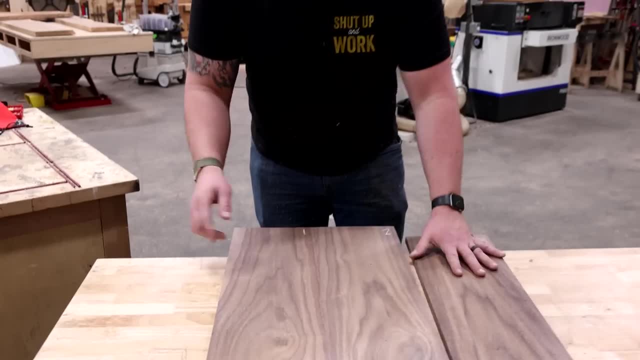 So here's the trick: When you're gluing these boards up, the only thing that matters is the angle on this face to this face. Okay, If I bring these two boards, one and two, together like this, I can joint this whole. 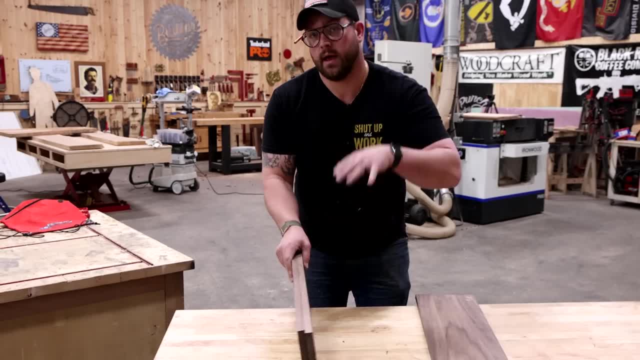 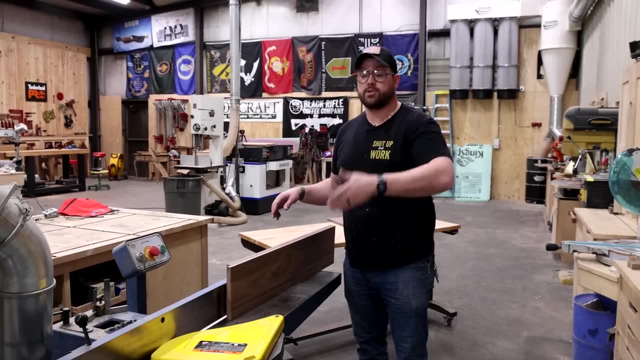 piece right here at one time and it'll give me a perfect joint, because they're going to be reflective of one another whether they're in or out. anyway, I'm not going to join them at the same time because some might say that that is unsafe. 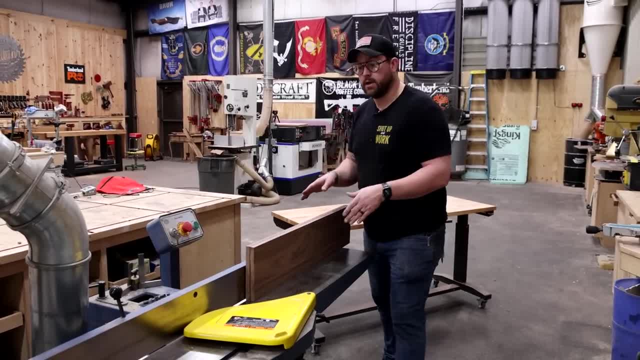 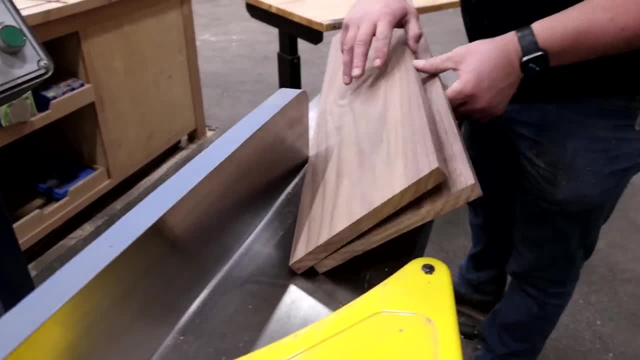 What I am going to do is make sure that I'm referencing the fence the same way. So remember our fence is out of square, We know that. But I'm going to have the back of board 1 against the fence and then the face of board. 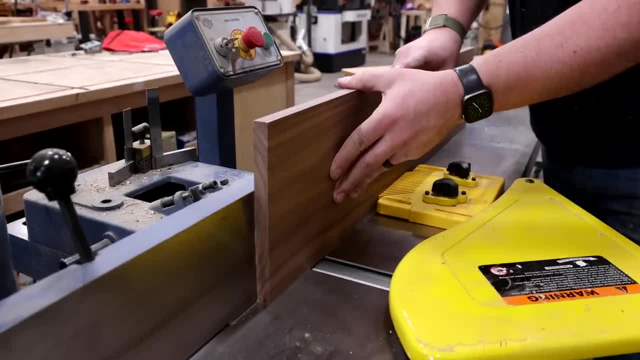 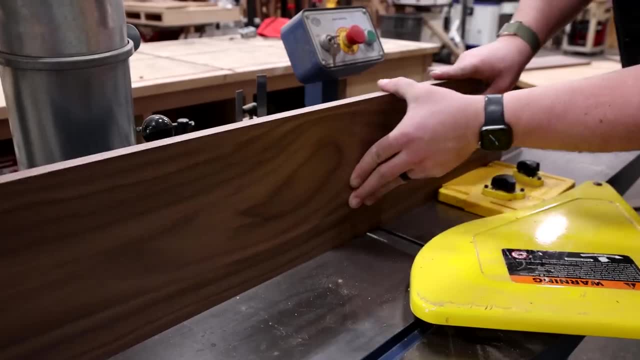 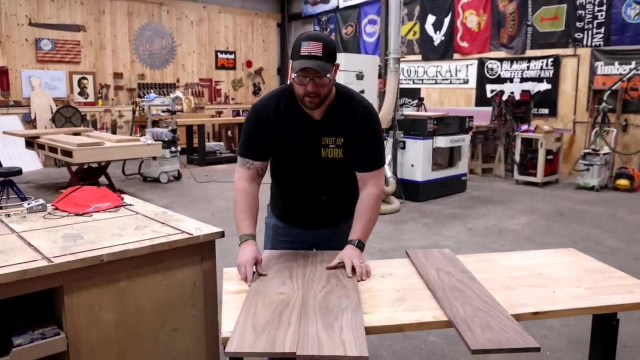 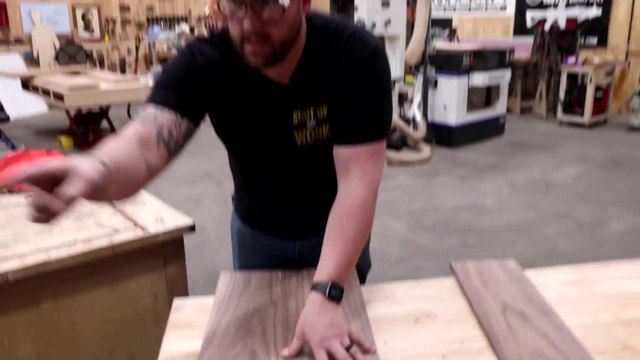 2 against the fence. Now, when these come together, they're going to look like this: See how pretty they are. As you can see, that joint is perfect And I showed you that on my jointer. the fence isn't square. 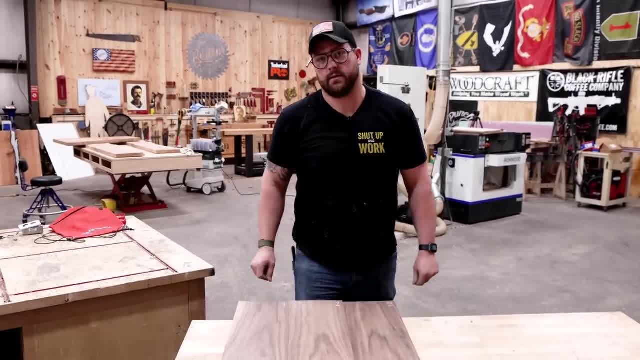 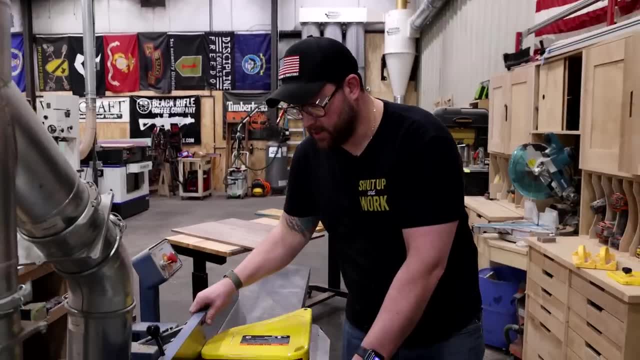 And when I learned this trick, it made my panel glue-ups look so much better. And while we're at the jointer, here's a bonus tip. I have a 10 inch wide jointer, but my first jointer was six inches. 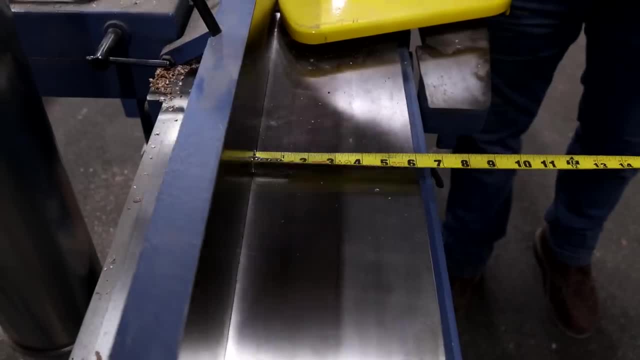 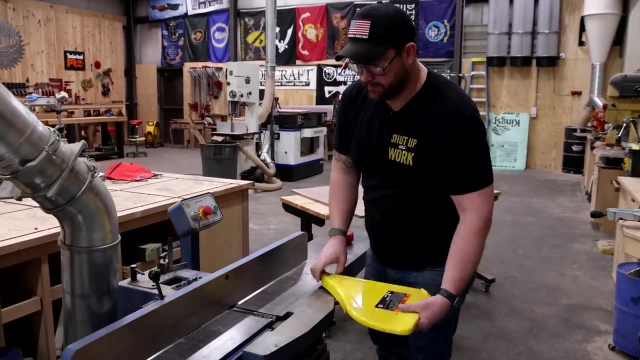 So what I'm gonna do is I'm gonna shrink this down here to six and I'm gonna show you guys a tip for doing boards wider than the width of your jointer. First you're gonna wanna remove your fence And we're doing what's called a face joint here. 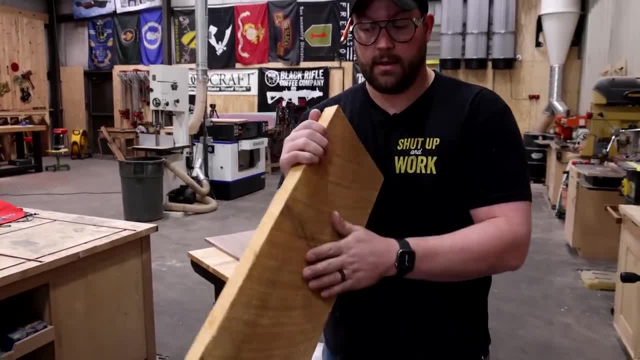 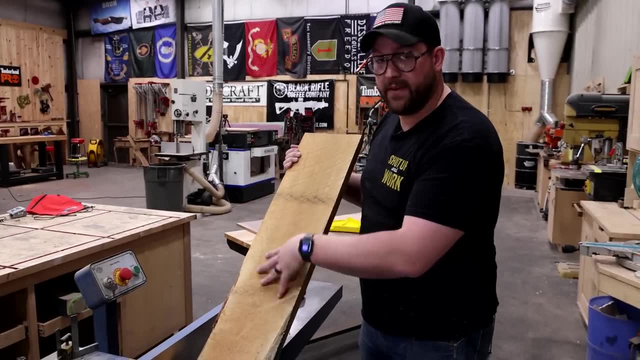 If you're not familiar, this is the face of the board and this is the edge. In order to get a square board, you have to prepare both of those. We're focusing on a face joint right now. Our board, as you can see, is only going to cut. 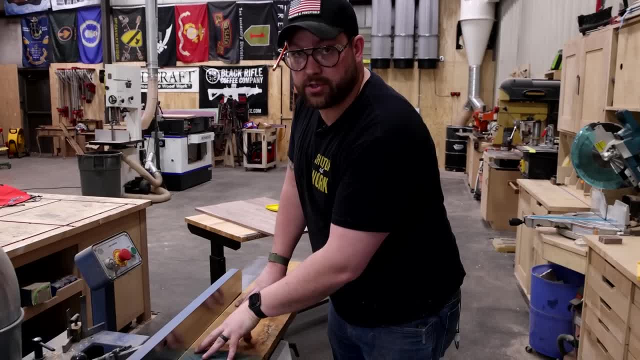 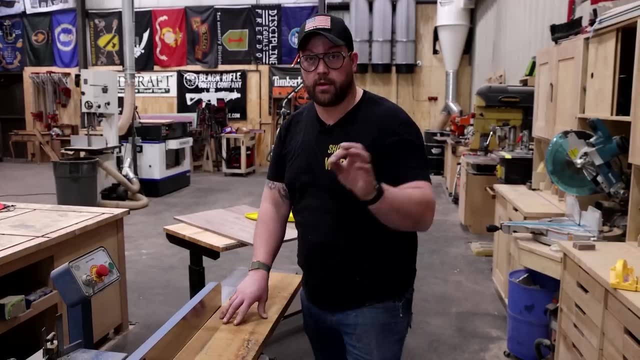 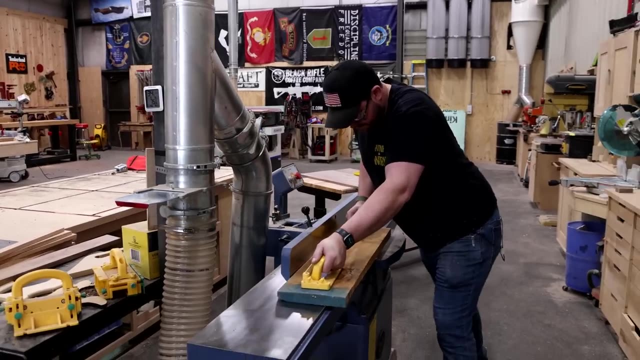 and leave an edge on this side. So we're gonna face joint this board and then I'm gonna show you our previous tip and a tip with the planer on how to make this board, This board, perfectly square and flat still. So you can see here, the jointer left a lip. 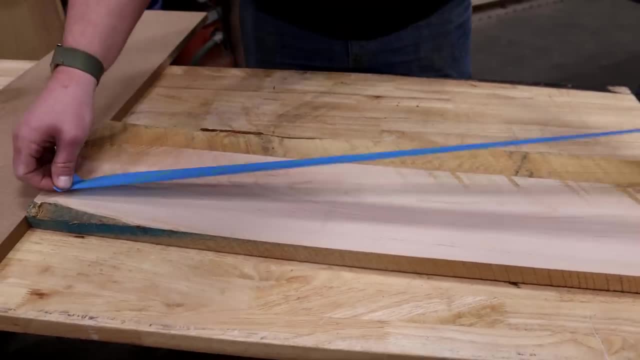 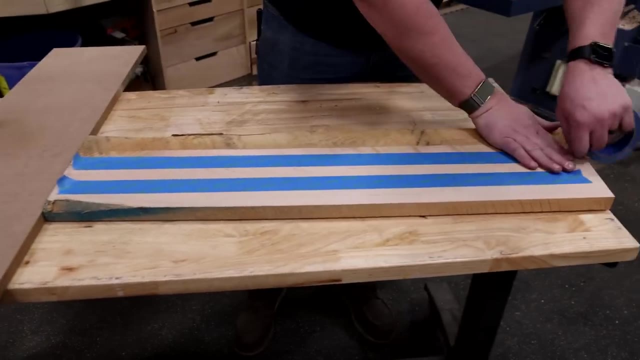 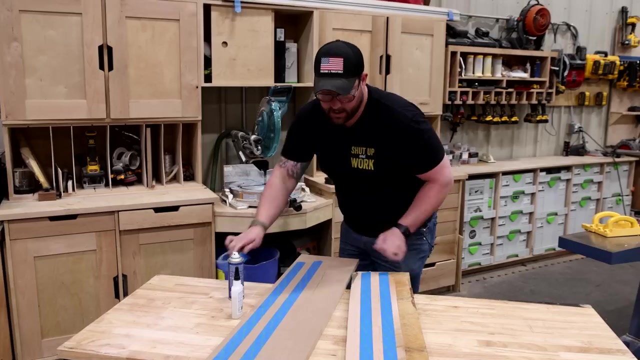 So what we're gonna do is now mount this piece of wood to something that's perfectly flat, like this MDF here, And I'm gonna use the exact same double-sided tape trick that I just showed you guys. There we go. Now these two are mounted together. 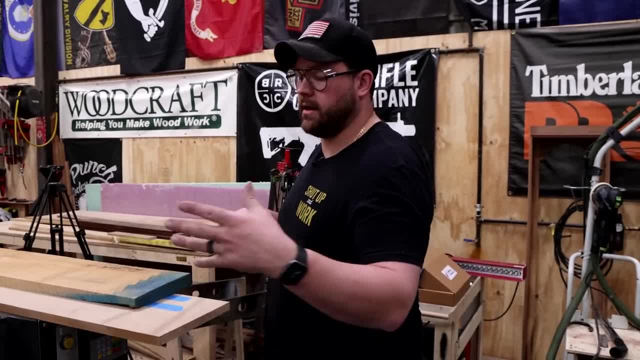 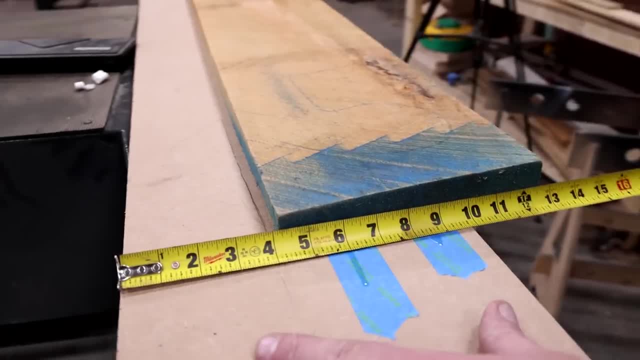 The next thing you need is a planer. Something important to note is that I have a super wide planer, but if you only have a 12-inch planer, you wanna make sure the overall width of your board and your sled are under, whatever the width. 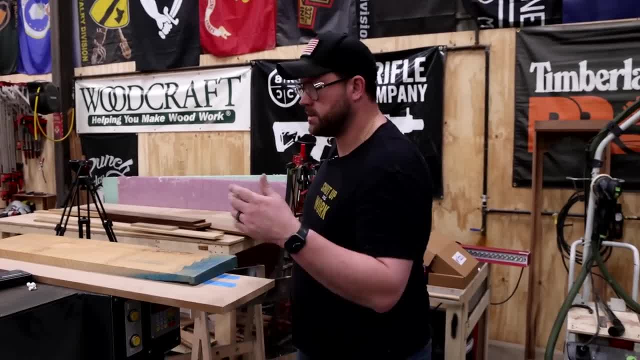 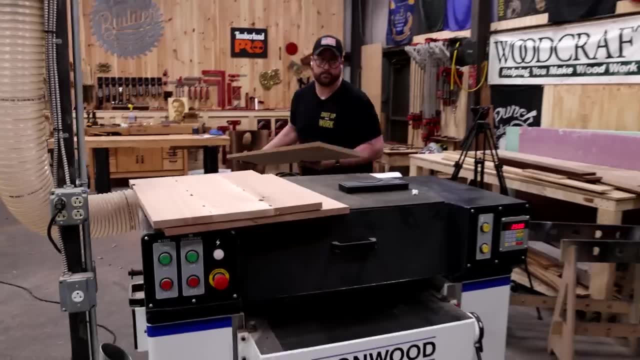 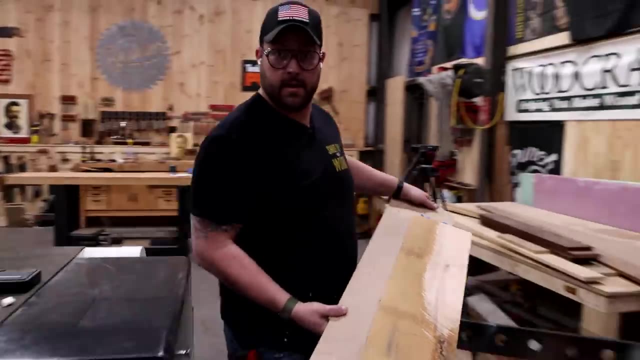 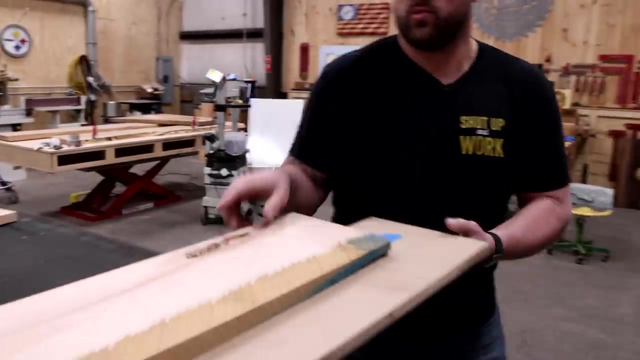 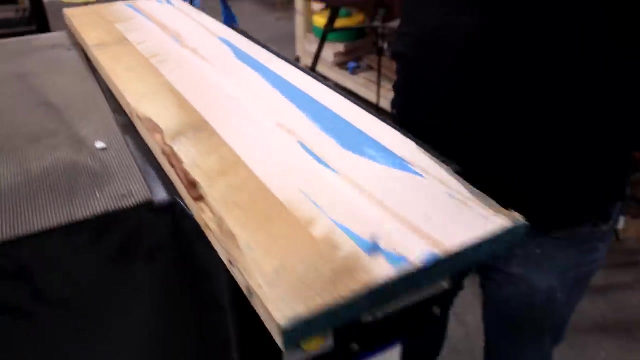 of your planer is. Most planers nowadays are up to 13 inches. Now all I'm gonna do is run this through the planer. give myself this flat side. See Now, we just pop it off. We run it back through. 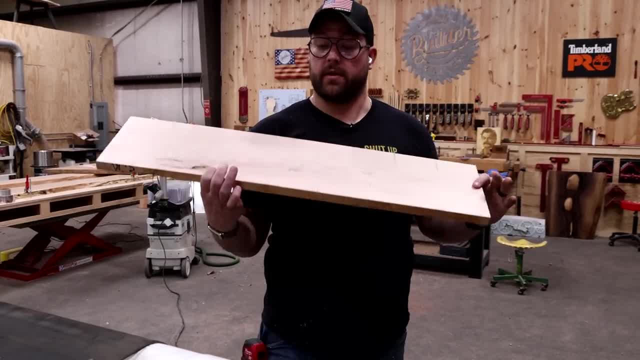 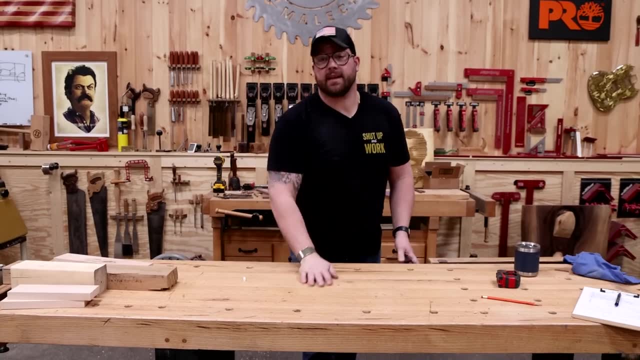 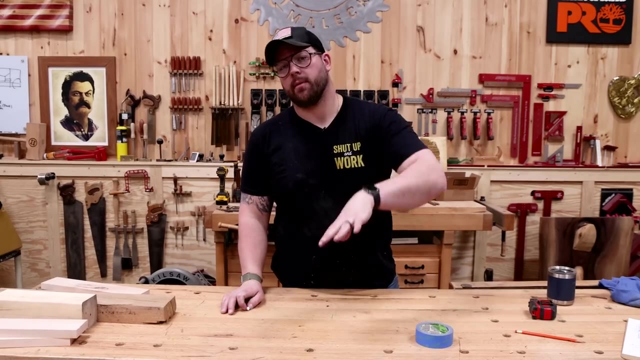 and just like that you have a perfectly flat board bonus tip. the fourth tip or technique that i wish i knew when i was getting started was using blue tape to help me with layout. now, if you've watched my content for a long time, you've probably seen me. 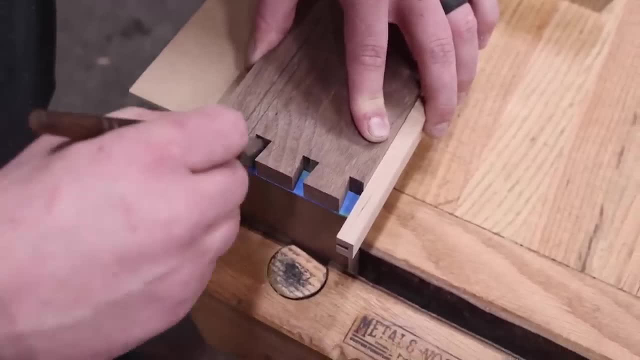 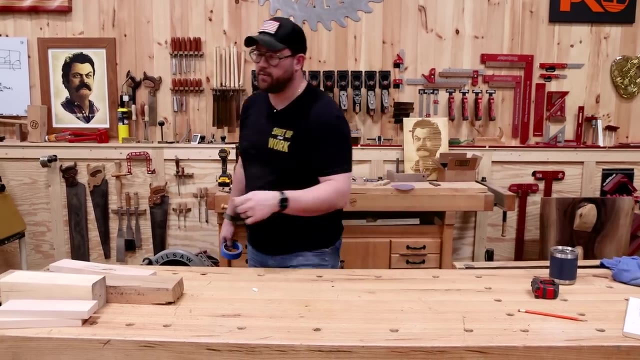 bust out blue tape to cut dovetails and to do some basic joinery, but this is, like i guess i don't know- one of the most abundant opportunities to use blue tape in the shop. let me show you a few examples here. let's act like we wanted to cut a mortise in this block right here. if i was going. 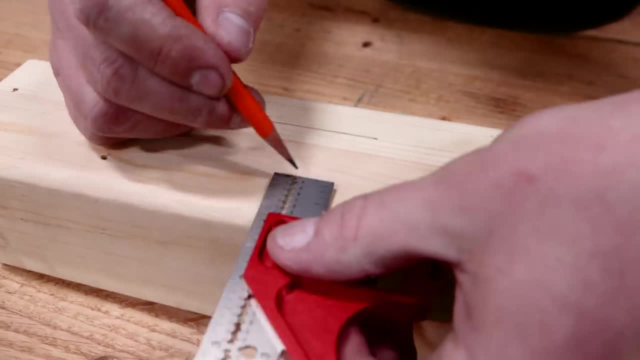 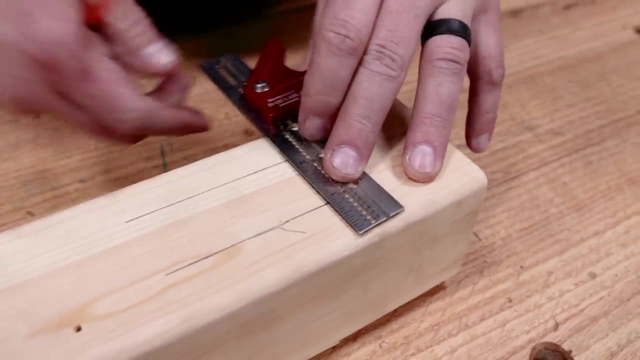 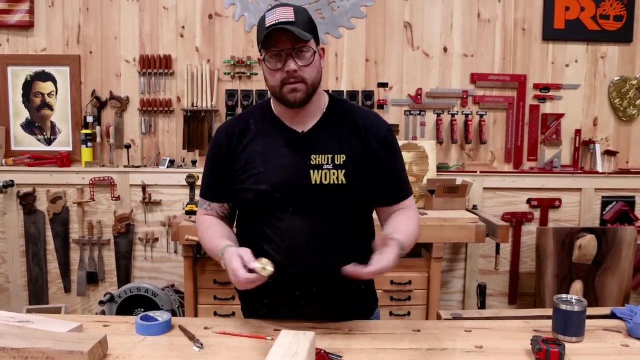 to do that, i'd probably initially establish the width of the block. let's just make our mortise one inch from each side. okay, now how long do we want to make it? let's just say we'll make a three inch mortise traditionally. what would be the next steps as a woodworker is: you'd want to come in? 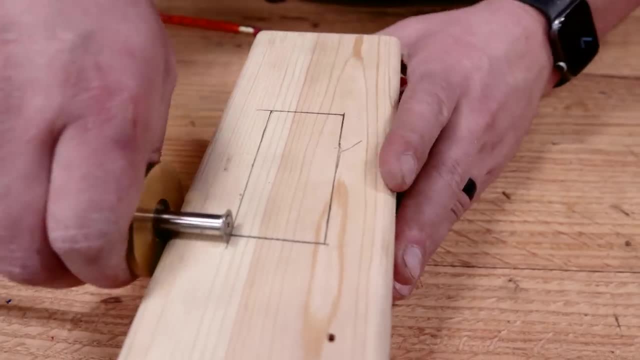 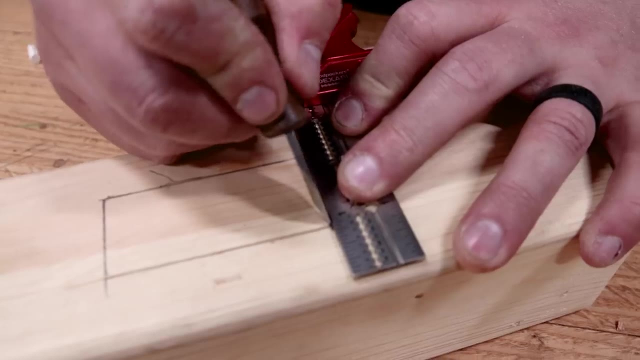 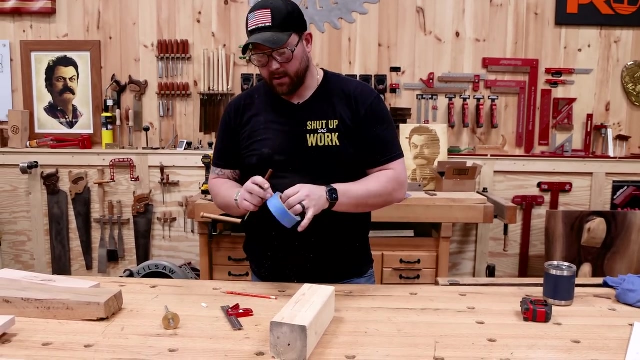 with your marking gauge like this: set it to that line. you come in, you mark it, flip the piece, mark it, then you come back, mark that end, mark that end and then you're going to go and start mortising out the material. but here is how i've started to adapt and do it. 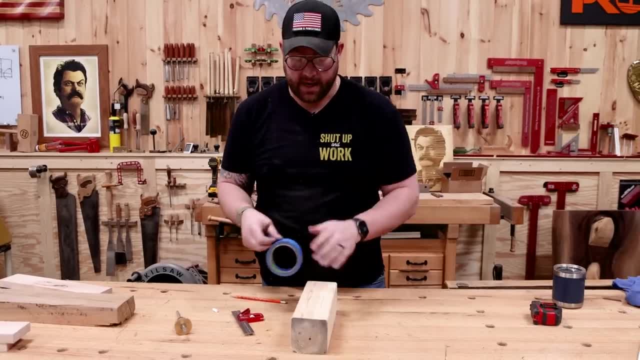 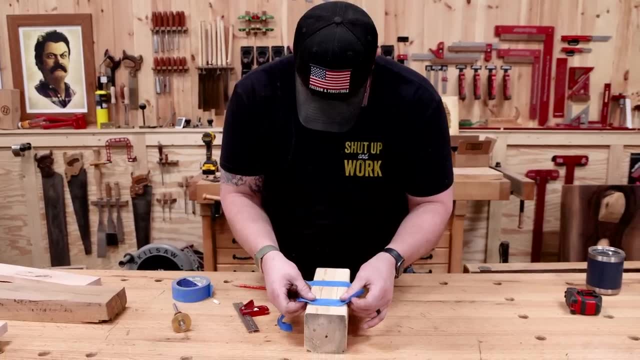 that, i think, just makes it so much easier. you're going to do the same technique. i'll come back and what i'll do is i'll put blue tape right on that line before i start cutting. i'll do the same thing on the other side. then i'm going to put a piece on this side. 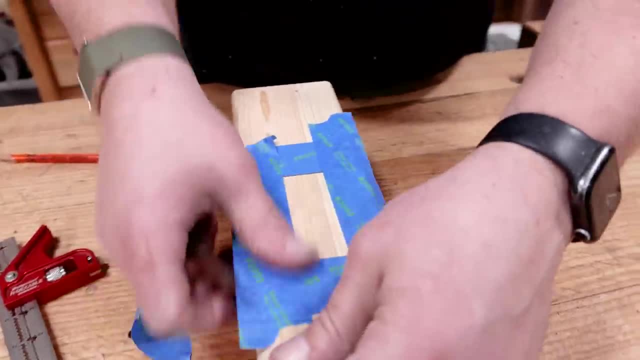 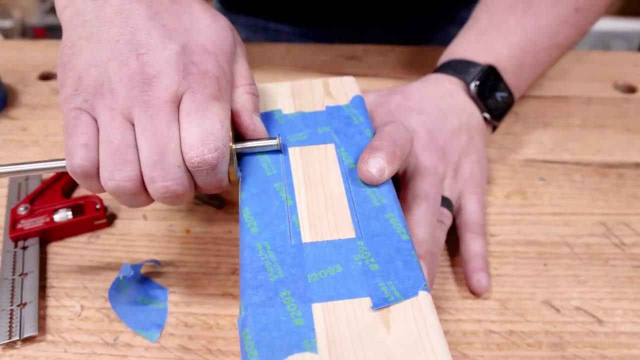 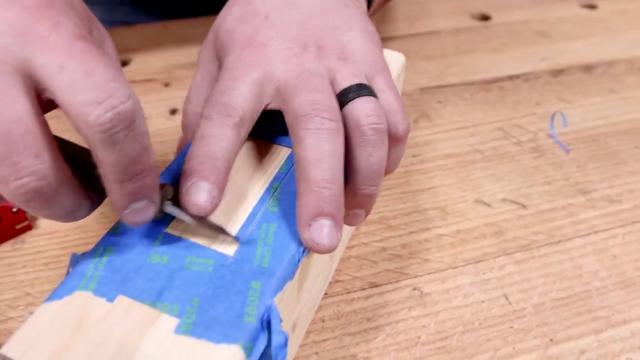 i don't care if it matches the line and a piece on this side, and i'll come back with that same marking gauge. i'll mark that line. i'll mark that line now. we already established that we're going to have that line underneath, so and we'll pull off from here and now. what we have is a much. 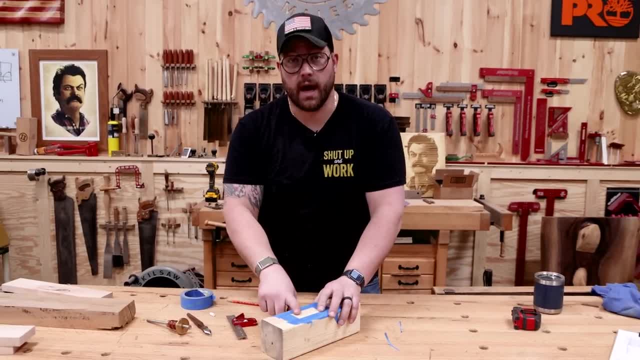 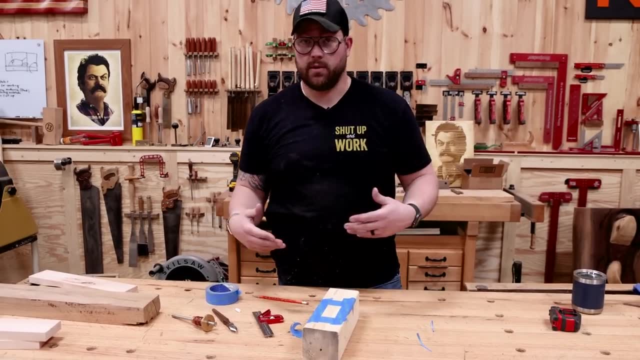 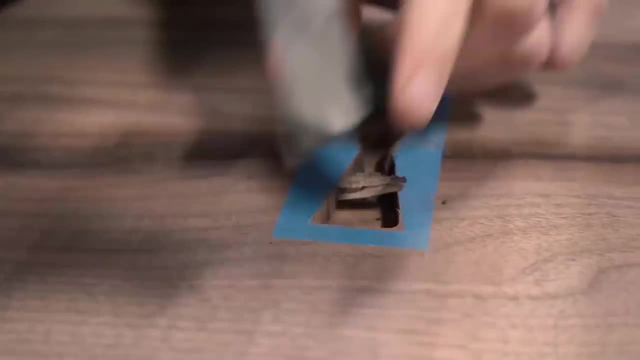 clearer representation of where we are cutting. the blue line is so much more of a difference in the wood. you can go about whatever method you prefer, whether you want to take this out with forstner bit, with a router. you guys have seen me hand cut bow ties into a lot of my work. i use this. 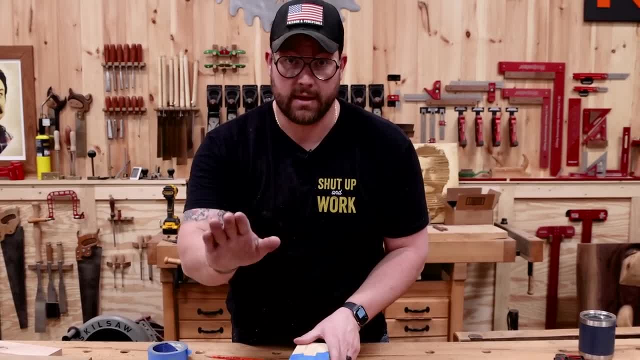 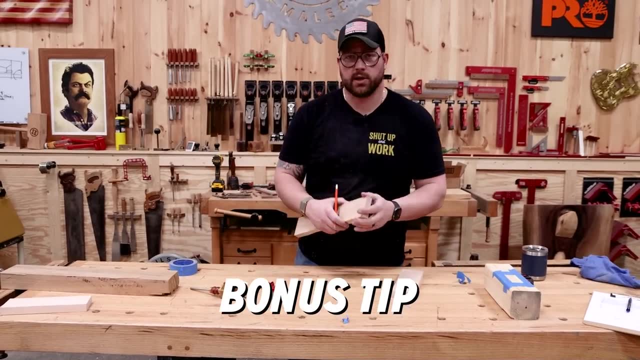 exact same technique works amazing in this application. i highly suggest it. you get way, way, way, way way cleaner results. but what if we want to cut a joint? well, here's a good example. say, i want to cut a dovetail joint on this piece of wood and then scribe it over here to this one. 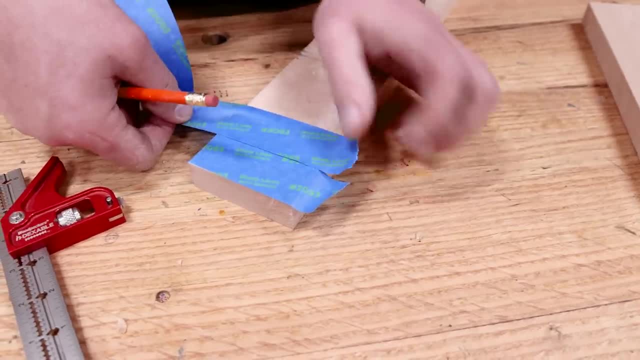 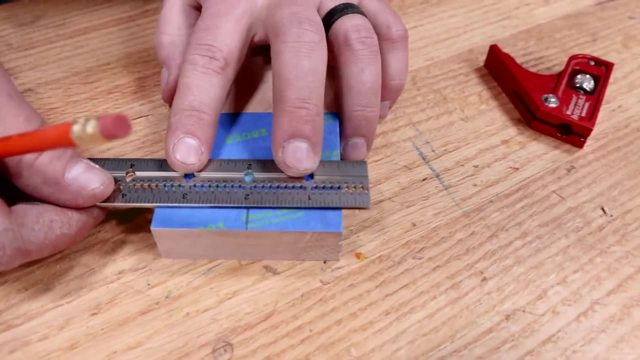 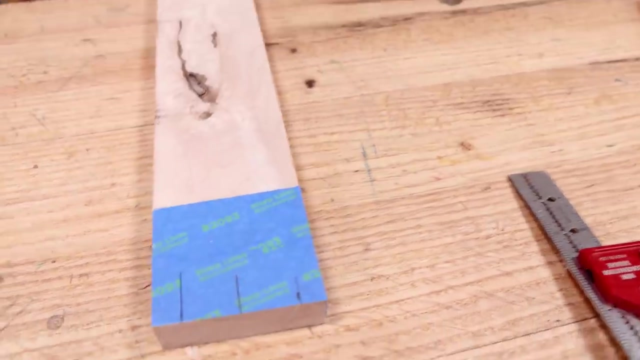 set up my blue tape on the edge of this board where i'm going to be cutting the dovetailed, more or less lap joint. okay, find center. we're going to measure ourselves an inch out on each side. there we go- inch. awesome. so this board's three inches wide. i'm going to set the depth of it to two inches here. 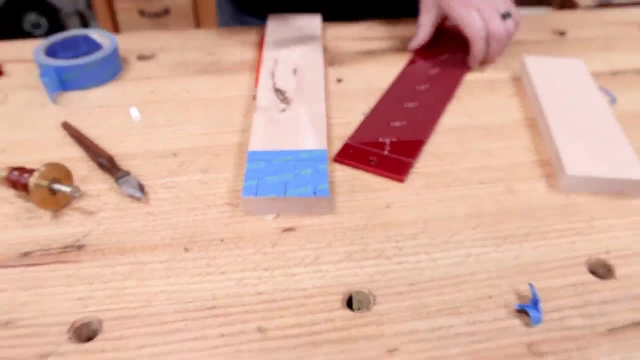 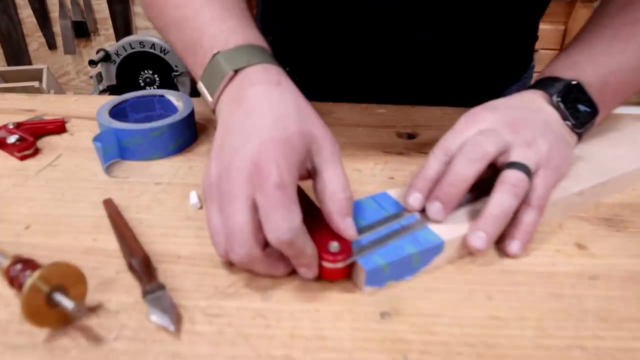 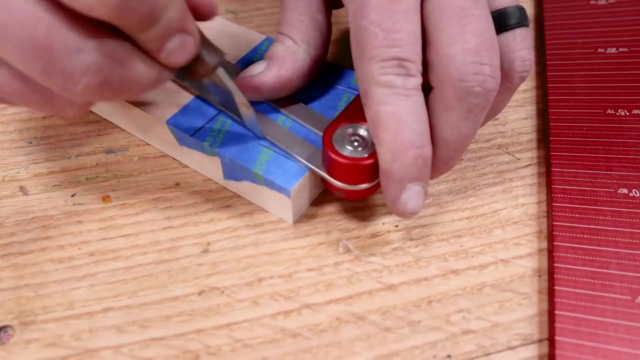 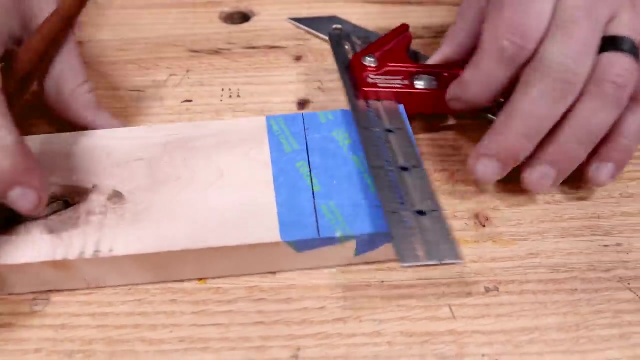 now i'm going to take my bevel gauge, i'm going to set to seven degrees. now i'll come in here. you're going to take that same marking knife now. cut that there. come back other side. we've got our point here and our point here. fantastic. so you always want to leave the blue. 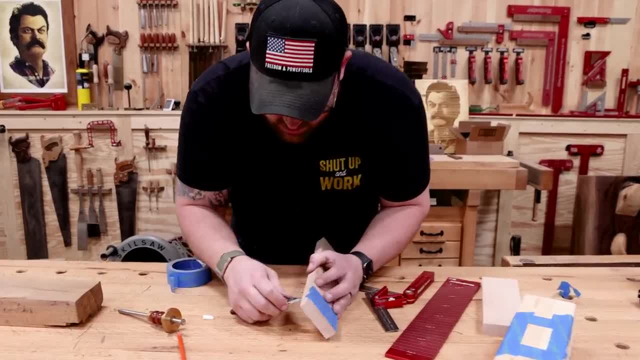 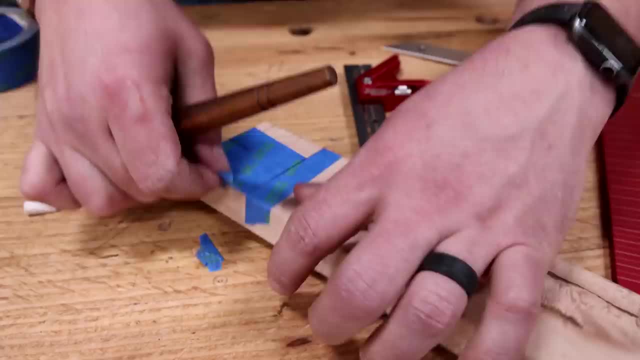 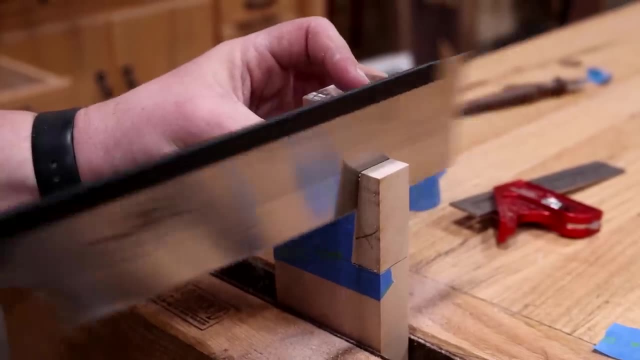 on the part that you're keeping. so for me, what this has done, it's really changed my ability to visualize my joints, because i'm going to remove the blue tape. i'm going to be able to perfectly see the part that i'm cutting, perfect. i can come back and make that perfect if i want. 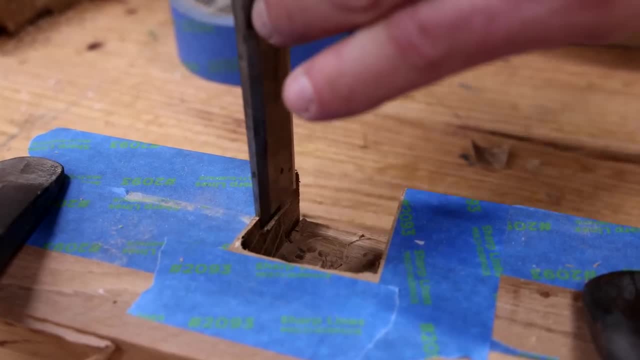 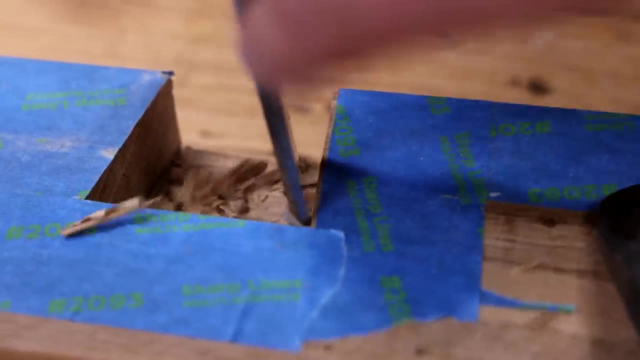 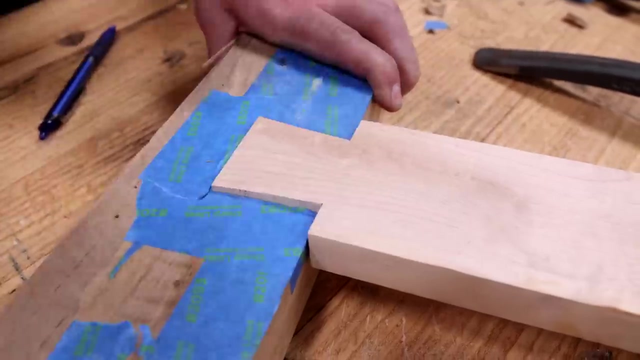 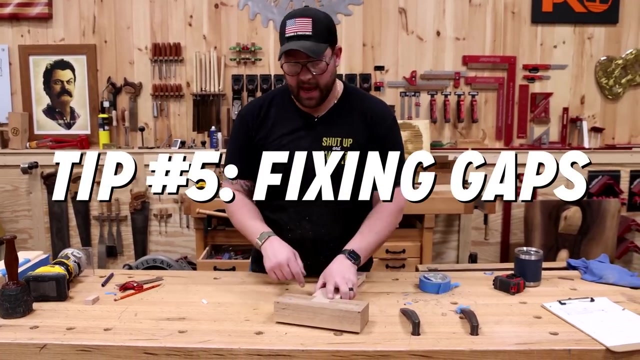 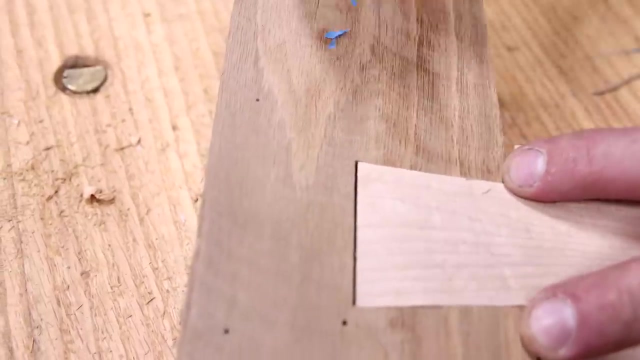 all right, so come back in over here. so for a pretty quick joint that's not that bad. but say you have gaps, just like these ones, because none of us are perfect. so you're looking here and you're looking here. well, when i was getting started i thought the only solution. 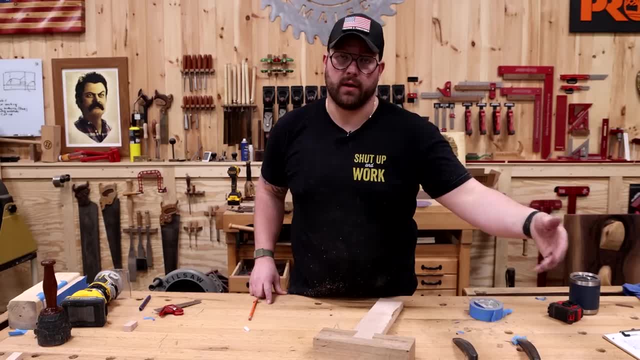 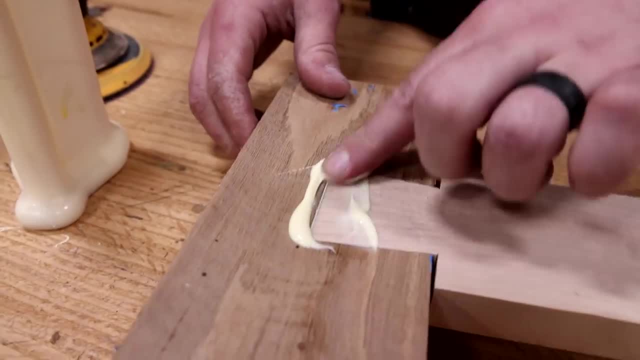 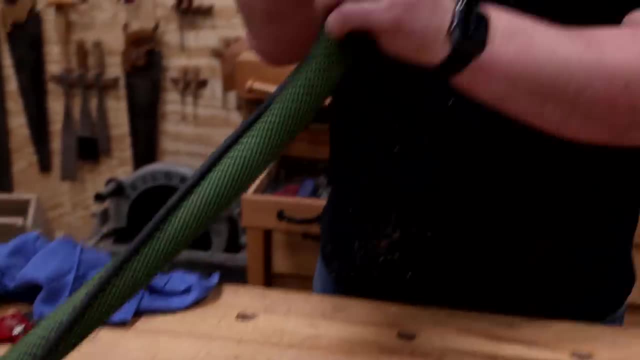 for that was to be better. or use wood filler. you don't need any wood filler. a better option for gaps in your glue ups is simply going to be putting some glue into the joint. that was an excessive amount of glue, but i want you guys to be able to see it on camera. unplug the dust hose, okay. 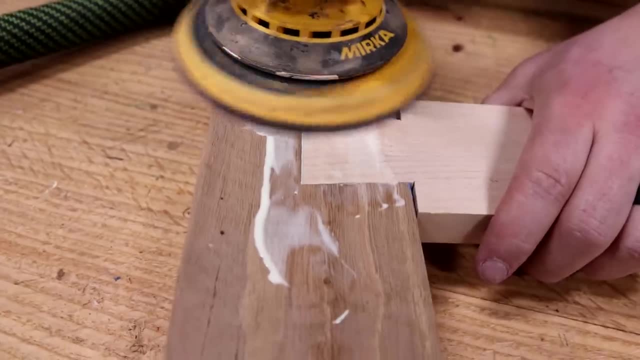 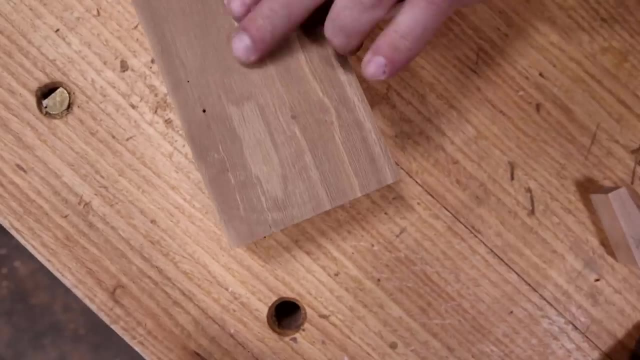 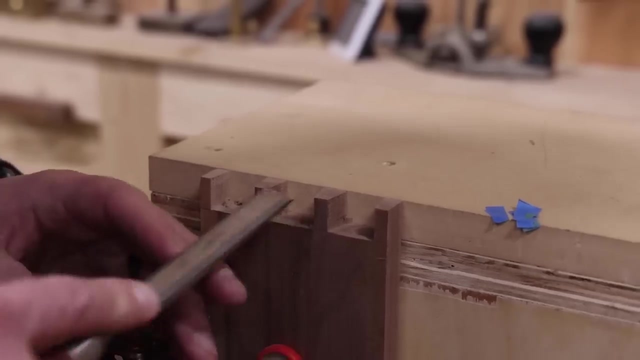 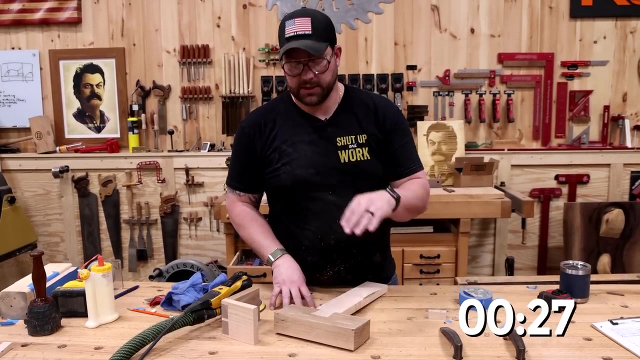 and just sand away. i use this technique on dovetail joints. i literally just used it on the three levels end table i built for the boxes. it just makes it look way more seamless. i wish i knew this when i was getting started, because it's such a simple fix, such an easy way, and it keeps the uh sand dust. 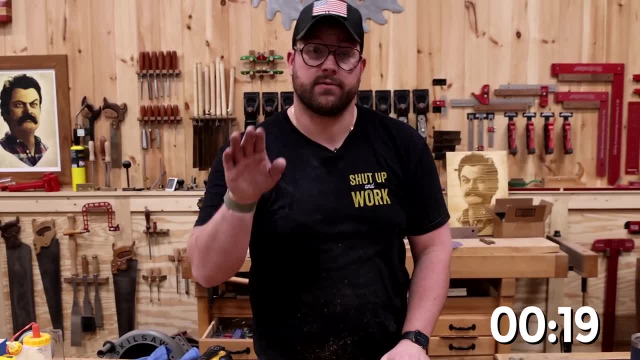 the same color as the wood filler, so you don't have to do the same thing over and over again. just sand the sand dust and stuff you know with the sand dust is easy to work with. and now i will advise this: if you're staining something, the glue won't stain, so just be aware of that. i don't stain.